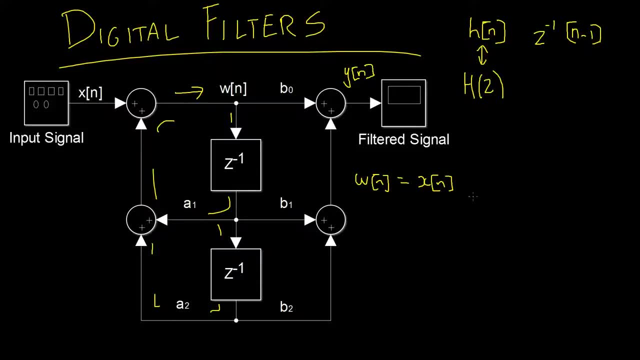 delay in the system. So how can we write that? if we have N, Well, we can do plus as it's being added back into the system W, because that's just a sample from one turn ago. Then we also multiply that by our scalar A1.. Then we also have this last loop here. so this one, So it's going to be X, our input, And this Z to the power of negative 1 is simply a one sample delay in the system. So how can we write that if we have N, Well, we can do plus as it's being added back into the system, W. 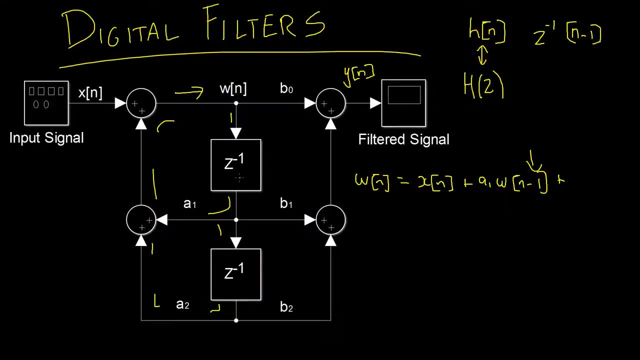 to take care of where there's now a 2-sample delay, as there's a minus 1 here, a minus 1 here, which will give us Wn-2, and then again scaled by A2.. Okay, so we've got our equation for Wn. Now let's take a similar approach. 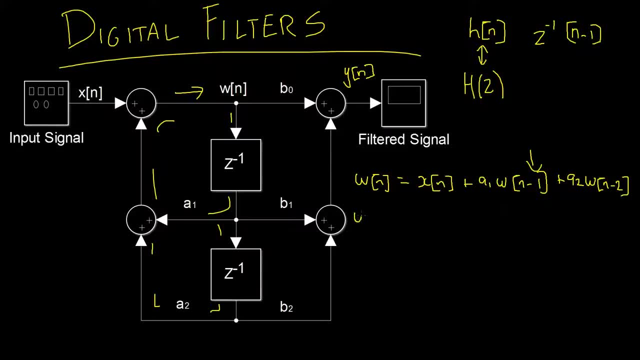 to calculate Y of n. First, we know Y of n is equal to Wn, which is entering this node here, and scaled by B0.. Then we also have the delay scaled by B1, and then we also have the double delay scaled by B2.. 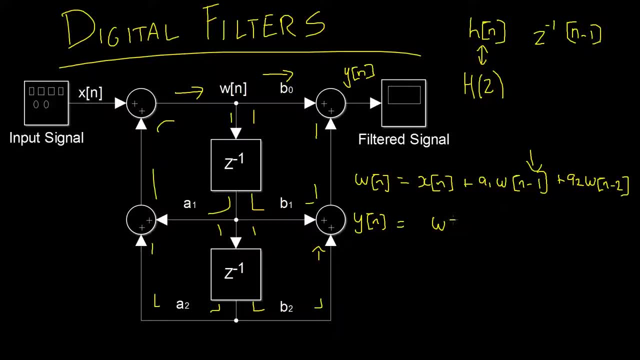 Just like before, we'll write that again. We have Wn and then that's scaled by Bo or B0, however you want to say it. Then we have plus Wn, and this time we're delayed by 1.. 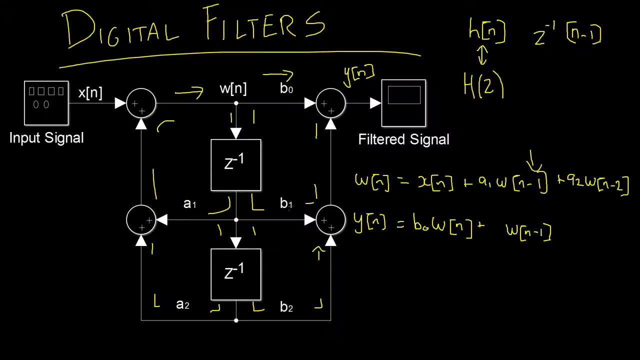 And then that's scaled by B1.. Plus our last loop Wn with a 2-sample delay, and then that's scaled by B2.. Okay, so we have our two equations, 1 and 2.. However, they're both in terms of n. 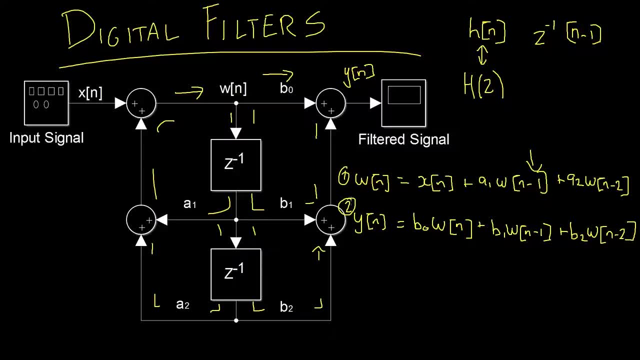 and we need them in terms of z. So what's the relationship between H of n and H of z? Well, as z to the power of negative, 1 is the same as a delay. we can replace all of the x of n's and w's of n's minus 1's and 2's. 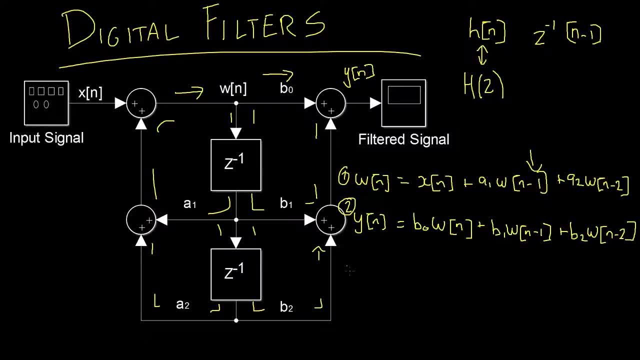 with x's and w's of z's. Okay, so our w of n becomes w of z, and then our x of n simply becomes x of- you guessed it- z plus our a1 remains unchanged: a1 multiplied by- you guessed it, z. 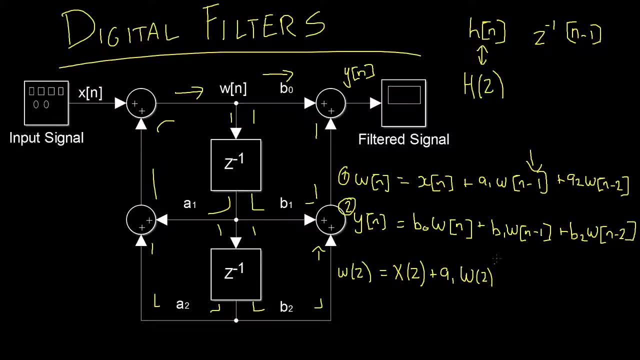 So we have our w of z and then times by our delay, which is simply z to the power of negative 1, because that indicates a 1-sample delay, And then to that we add a2 w of z and then z to the power of negative 2,. 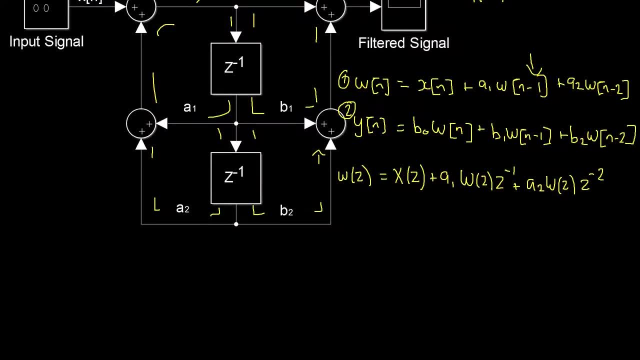 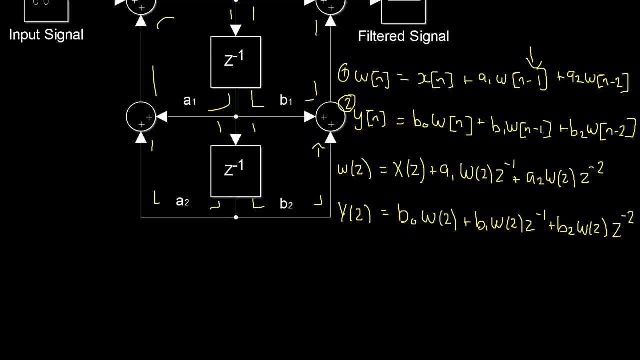 because in this case it's a 2-sample delay. We can repeat this process for the y of n, which will give us: Okay. so we now have all of our y of n's and w of z and we now have all of the components that we need to calculate our h of z. 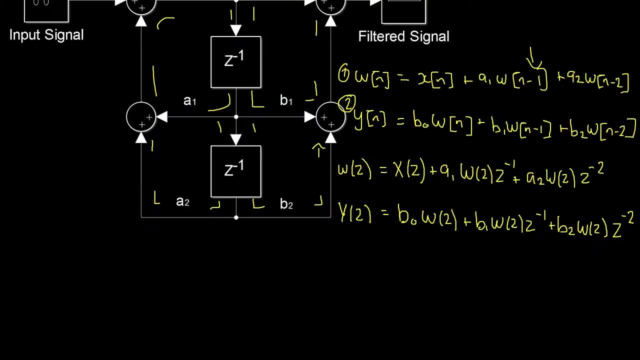 Okay, so we can isolate x of z by subtracting a1 wz z to the power of negative 1 plus a1 wz z to the power of negative 2 from both sides of this equation. On the right-hand side we'll have w of z. 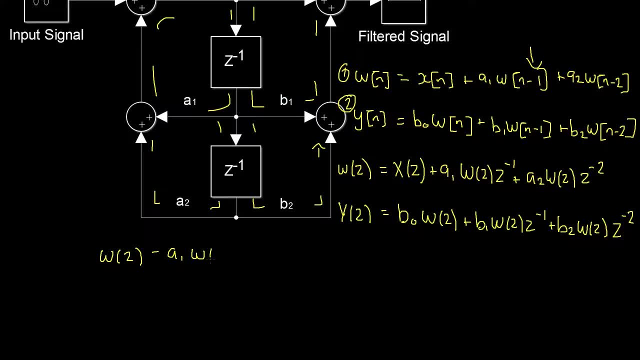 minus a1. w of z. z to the power of negative. 1 minus a2. w of z minus a2. w of z. z to the power of negative 1 minus a2. w of z. z to the power of negative. 1 minus a2. w of z. z to the power of negative 2. 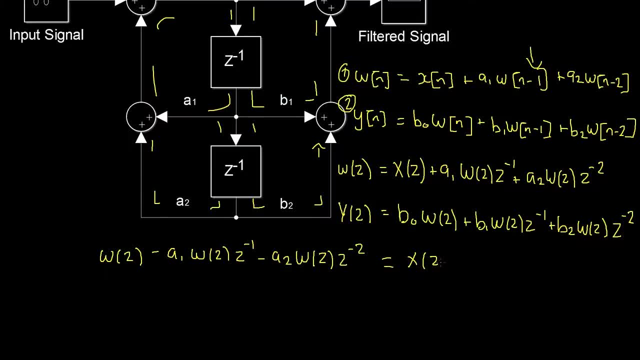 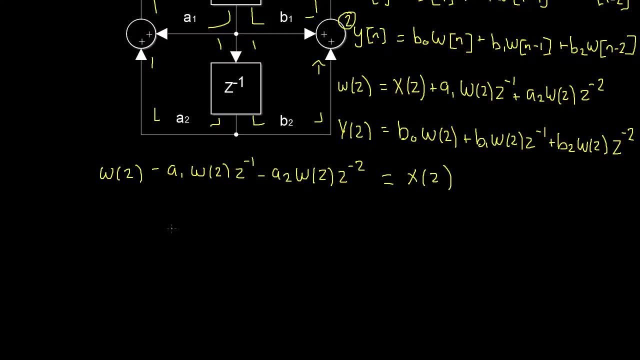 and that's all equal to x of z. Okay, so you might be able to notice that we have a w of z in all of our terms on the left-hand side. Why don't we bring that out the front of the equation? and while we're at it, let's flip the sides so that we have x of z on the left? 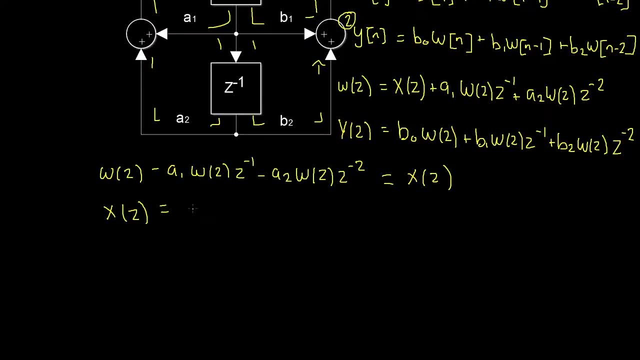 We'll have: x of z is equal to w of z outside the brackets, and then inside the brackets we have 1, because that will leave 1, minus minus a1 z to the power of negative 1, minus a2 z to the power of negative 2.. 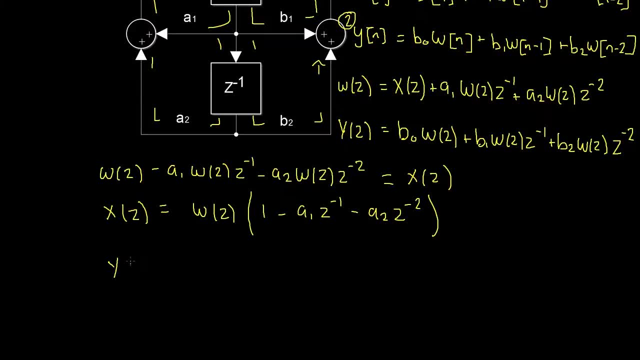 We can do the same with our y equation, which will give us: y of z is equal to w of z, and then, inside the brackets, b0 plus b1 z to the power of negative 1 plus b2 z to the power of negative 2.. 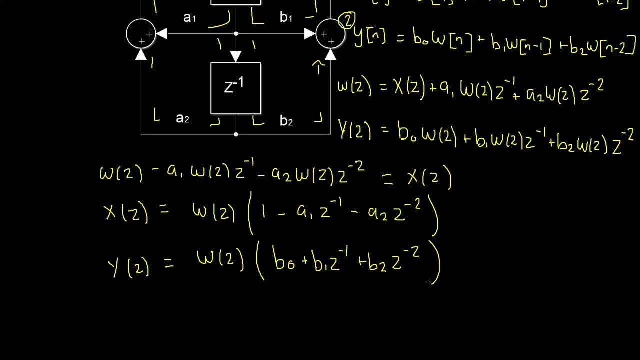 Excellent, so we're making a lot of progress. so we're making a lot of progress. now We have w of z in both of our equations and now we can cancel them out nicely to calculate our h of z. Let's do that now.